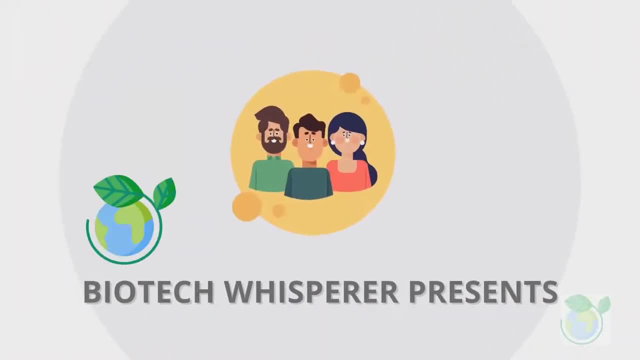 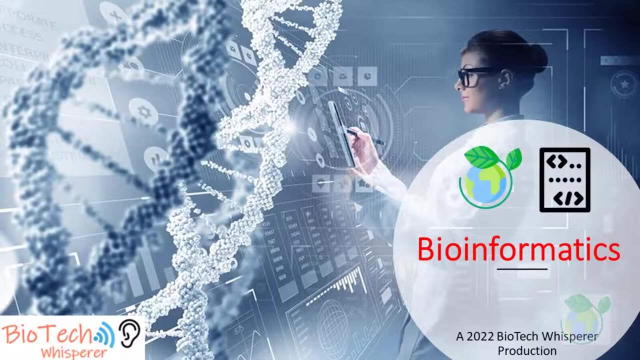 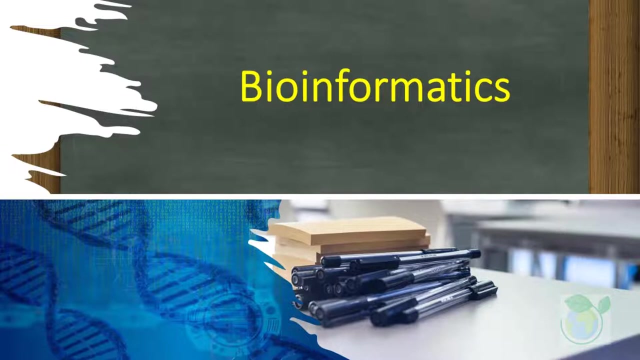 Welcome to the BioWhisperer channel. Our topic today is on a prospective overview of bioinformatics. If you are new here, we are a group of retired professors sharing bite-sized videos in life sciences. Let's dive into the topic for today. 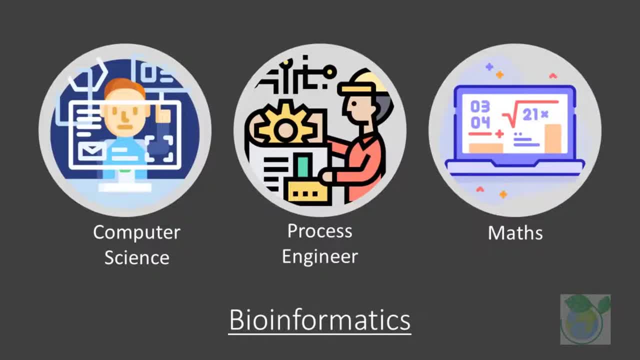 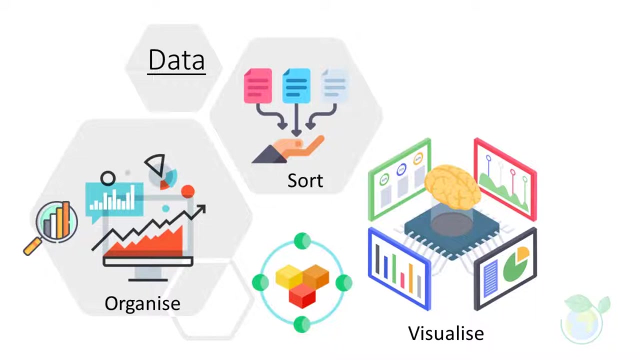 Introduction to Bioinformatics. Bioinformatics can be simply defined as an approach that uses computer science, engineering and mathematical methodologies to manage, visualize and analyze data, to discover new patterns and build hypotheses and models. The infiltration of bioinformatical biology may be more profound in shifting the biological research paradigm than molecular biology. 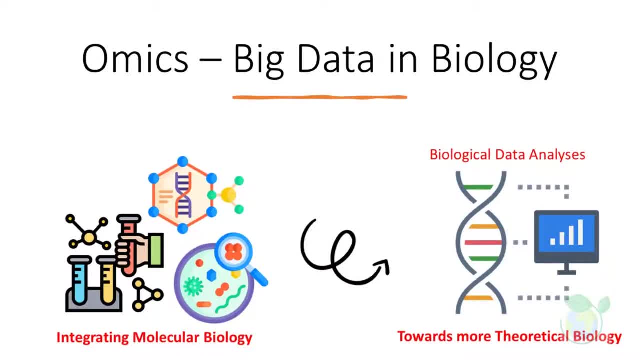 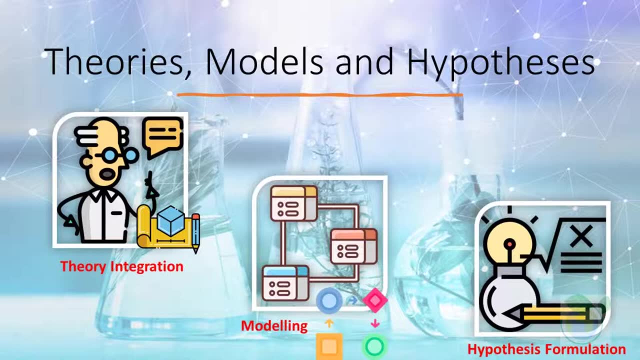 ever was. The richness and enormity of information, such as understanding the function of every gene in an organism, will shift research into a new field of research, into more theoretical biology, using bioinformatical approaches, with experiments carried out to find supporting or refuting evidence for the theories, models and hypotheses. 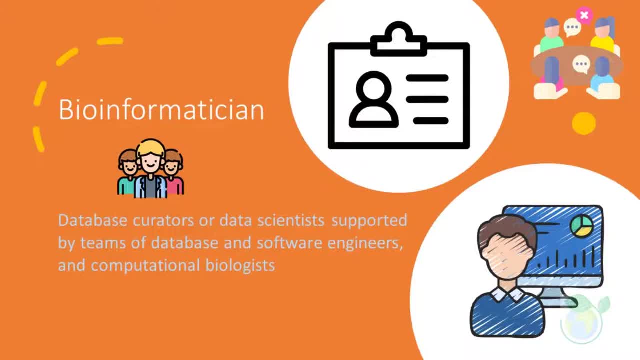 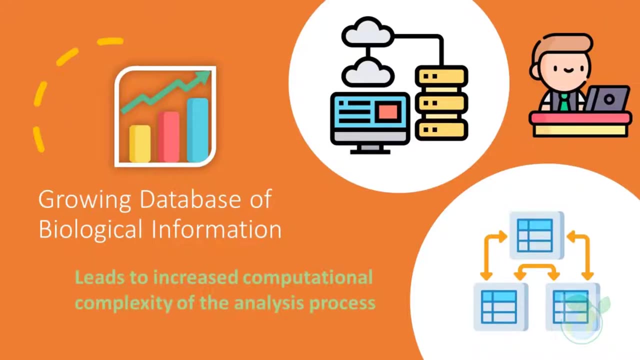 At present, bioinformatics is mainly conducted by a specialized group of individuals, such as database curators or data scientists, supported by teams of database and software engineers and computational biologists. The growing size of sequences, protein and other biological databases results in an increased 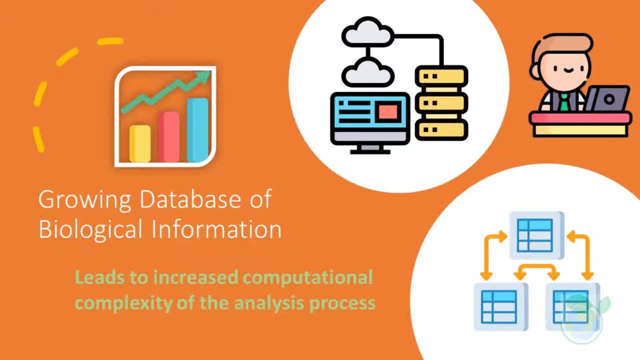 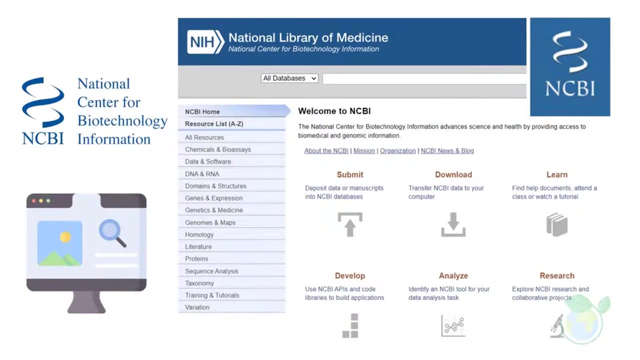 computational complexity of the analysis process. Often parallelization is the only solution to limit the turnaround time within reasonable limits. Platform-level tools are made available in the initial days of bioinformatics as web tools which are hosted at sites such as Exposy or National Center for Bioinformatics. 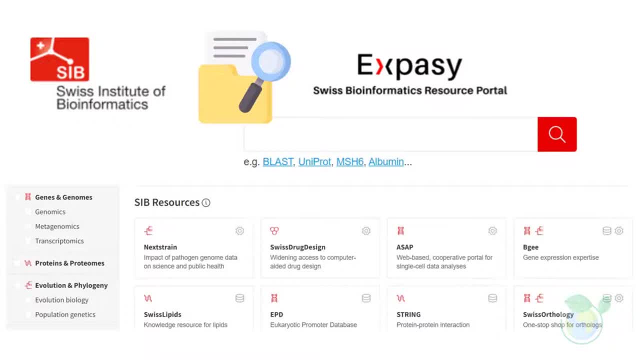 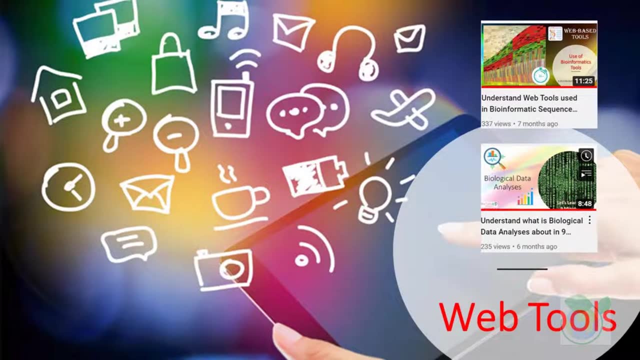 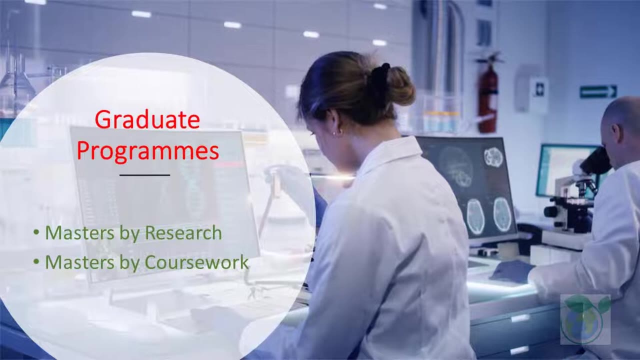 In fact, the majority of the biologists, graduate students, postdocs or research scientists are users of the most basic bioinformatical tools or web tools. Graduate-level bioinformatics programs at the master's level are gradually embedding programming, database development and management of large datasets and quantitative and statistical analysis of data into